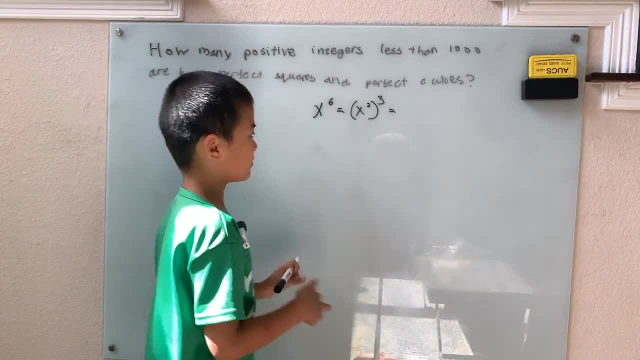 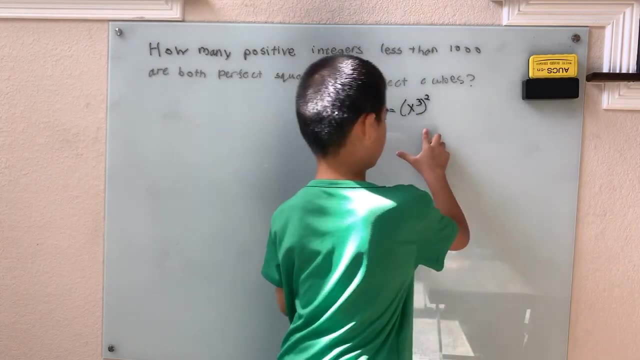 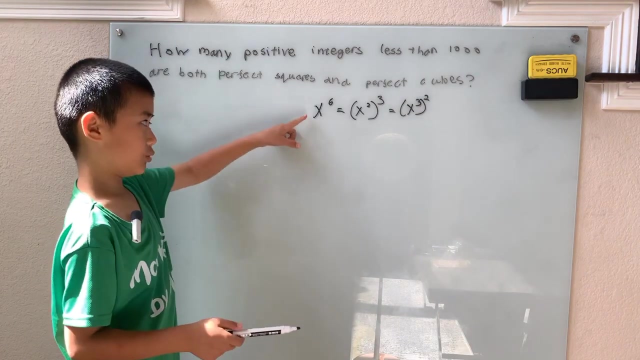 cube. Or you can write 6 as 3 times 2, and then power of the power rule, power of the power rule again, and you get x cubed squared. So both of these cube squared. That means every number can be written as x to the sixth if it is a perfect square and a perfect cube. 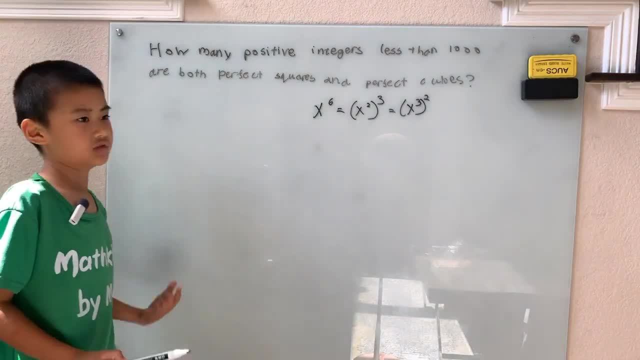 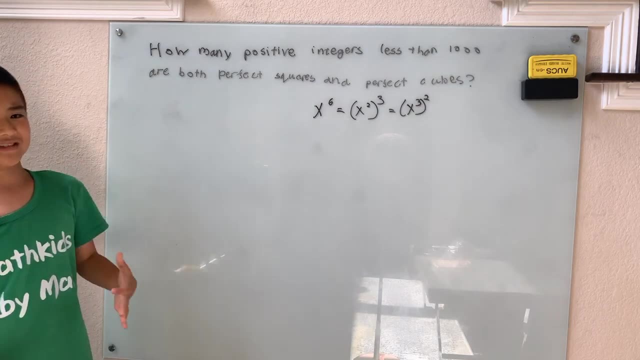 That means we can list out all of the six powers, less than 1000.. Of course they have to be positive and since I'm listing them out, I'm going to tell you six power sticks is really big for power that you want to compute, actually, since I mean. so there's really. 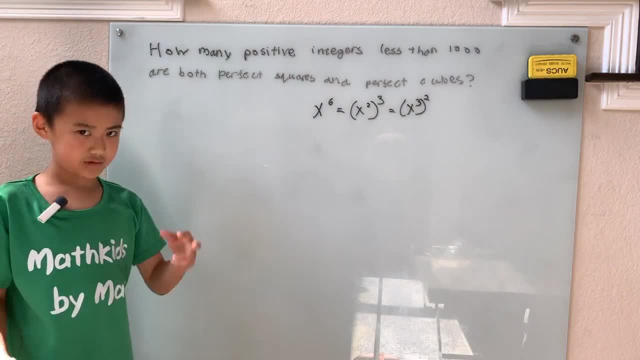 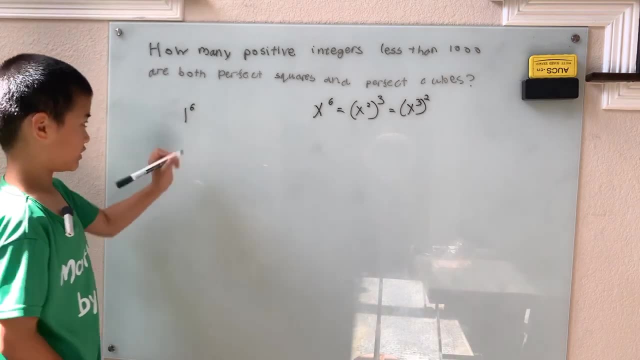 not a lot of six powers, less than 1000, which is a little small compared to the six power size. And you'll see why: because, well, starting with 1 to the sixth, which is just 1, definitely less than 1000.. 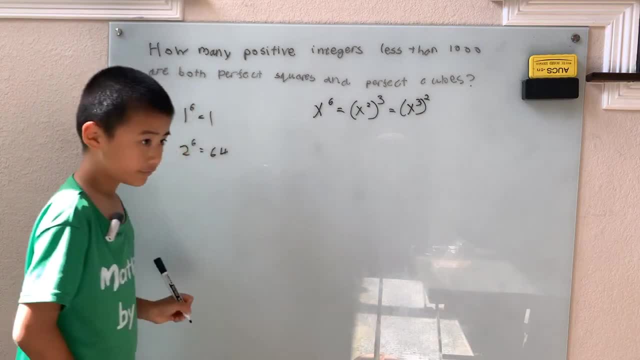 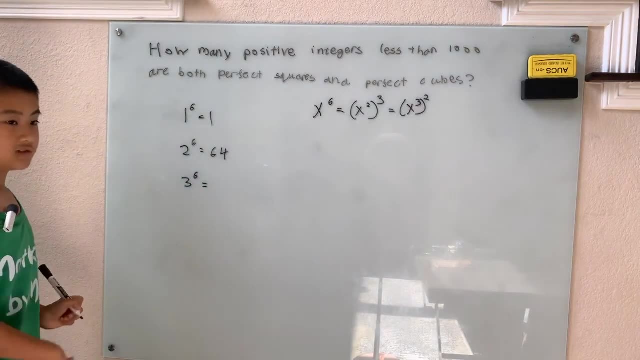 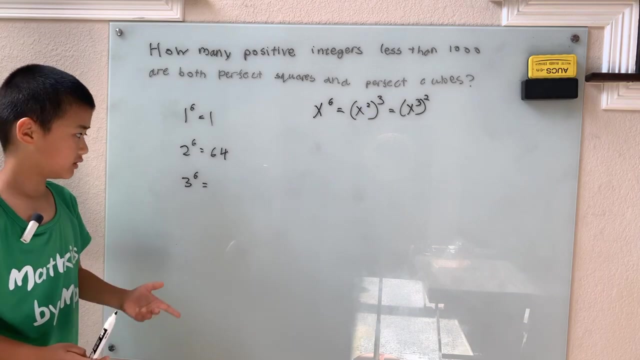 2 to the sixth is 64.. Well, we'll move on to 6, I mean 3 to the sixth, because 64, that's the less than 1000.. Now, instead of computing that, well, 3 to the sixth is 3 squared I. 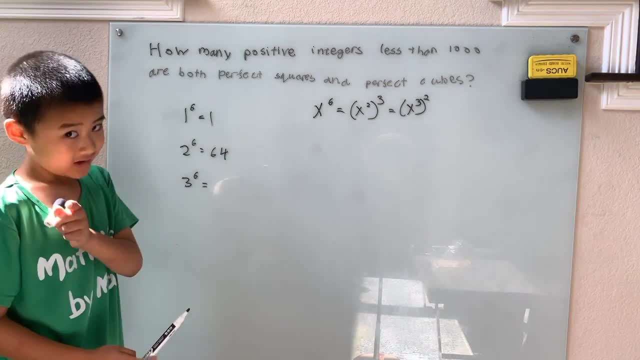 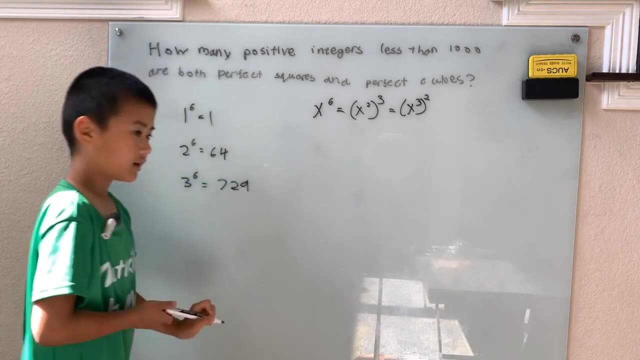 mean 3 squared cubed. 3 squared is 9.. And if you know your cubes, you'll know that 9 cubed is 729.. But if you don't, you can just flop that. I'll flip-flop this around: 3 cubed squared- 3 cubed is 27.. You can just multiply out 27. 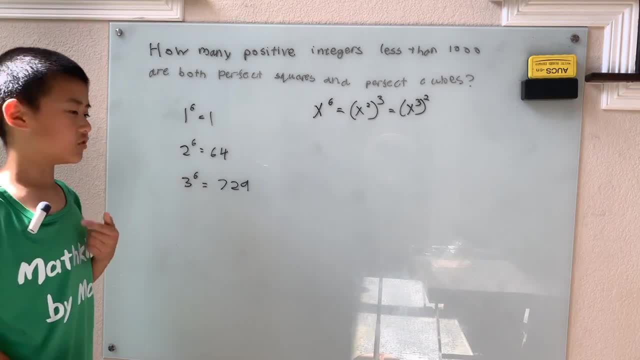 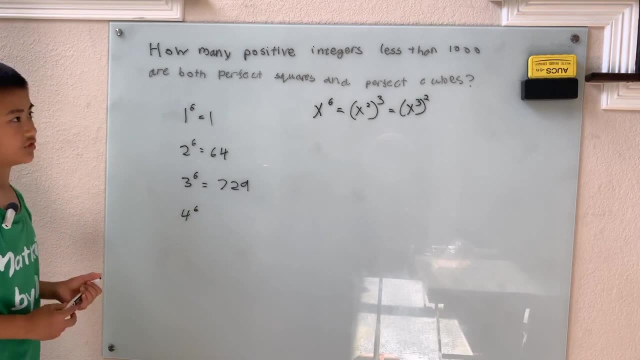 times 27 using the multiplication algorithm. if you want, that is Now, I'll move on to 4 to the sixth, And that's why I'm telling you there's not many six powers less than 1000, because 4 to the sixth is larger than 1000, because, well, 4 to the 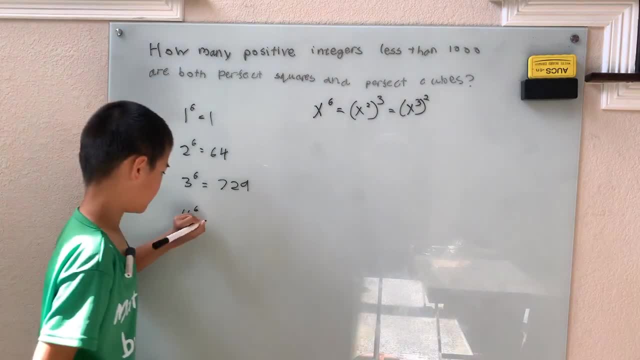 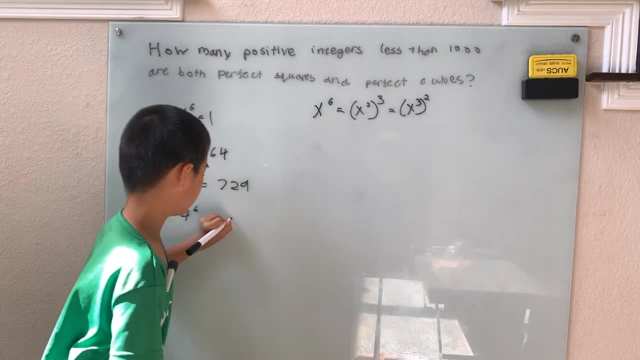 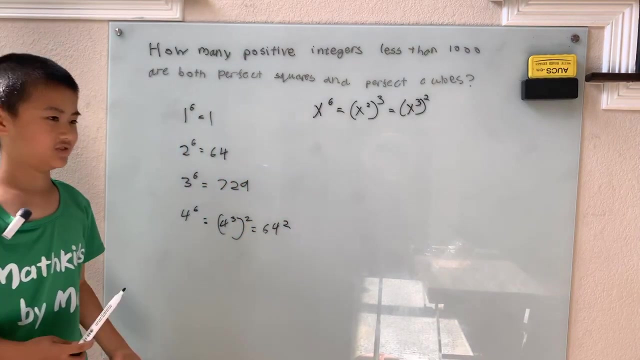 sixth: well, 4 squared. yeah, I'm just going to write down a little bit of math here to tell you This is, let's see, 4 cubed squared. 4 cubed is 64 squared. Oh, that's not good since. 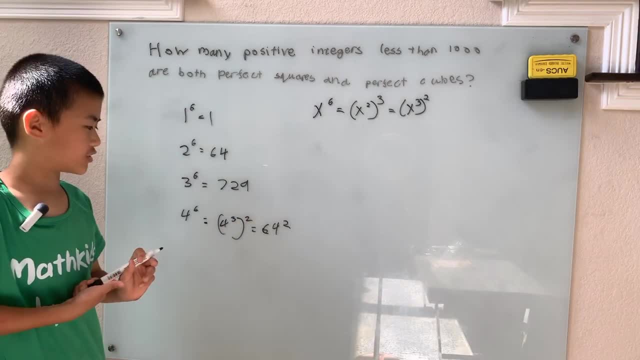 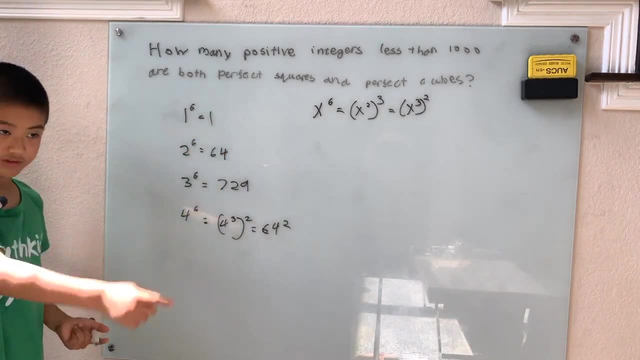 60 squared is already 3600.. It's going to be way larger. 64 squared is going to be way larger than 1000.. That means 4 to the sixth. well, bye-bye, That means there's only 1,.